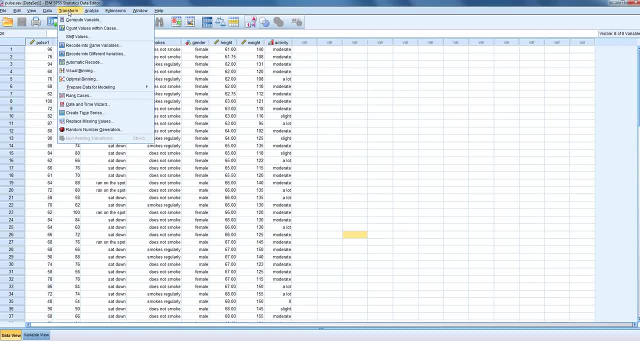 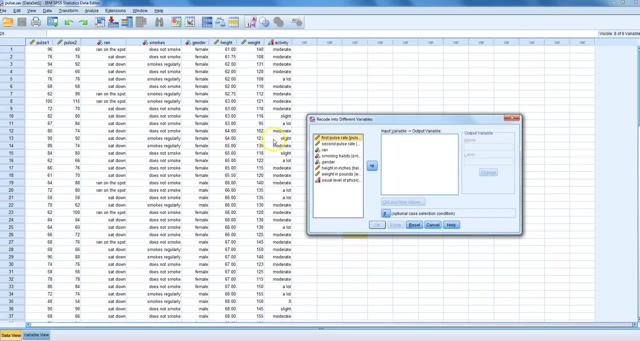 At the top, we select, transform and then recode into different variables. This is going to create a new column which will state which height group the person falls into. So we're looking at people's heights. so we need to drag height across to the right hand box. 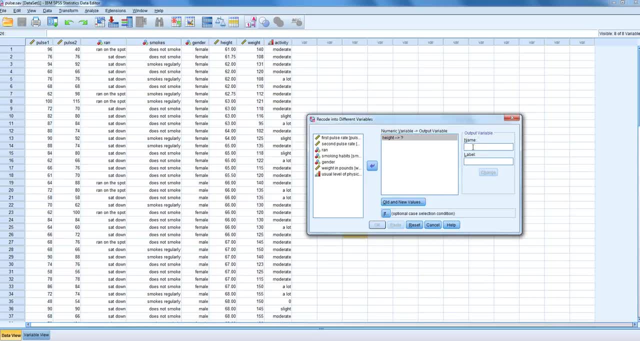 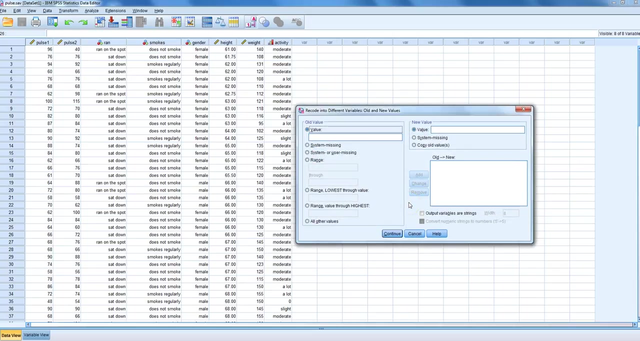 and we have to give our new variable a new name, For example height group. We select change. We now need to tell SPSS which heights go into which group. We select old and new values. We've said those at 64 and below are going to go into the small group, so we do that. 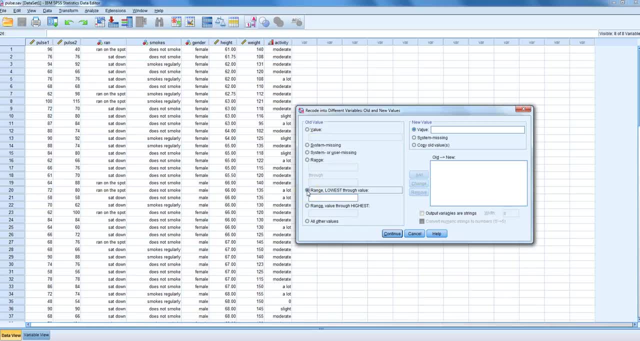 as follows: Select range, lowest true value and type in 64, and these are going to go into group one. We then select add. Now the medium group are between 64 and 72. So we select range and I'm going to select 64.001, because if I select 64, that also occurred. 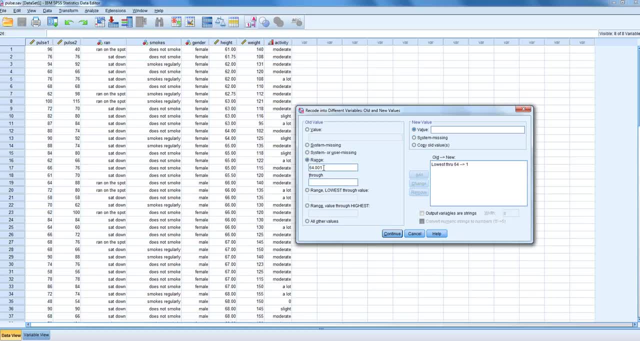 in the short group and then that means a person may go into both groups, which we don't really want, And the highest value of the medium group is 72, but again, I'm going to call it 71.999.. So the 72 people are in the short group. 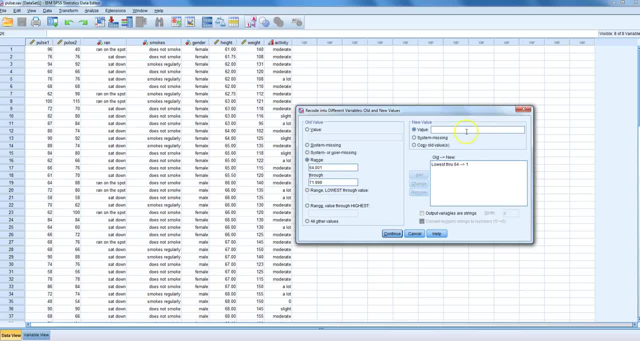 The 72 people will go in the highest group. This has a new value of two because it's the middle group and we select add. Then the tallest group are those 72 inches and above. We select range value through highest 72, and they're going into group three. 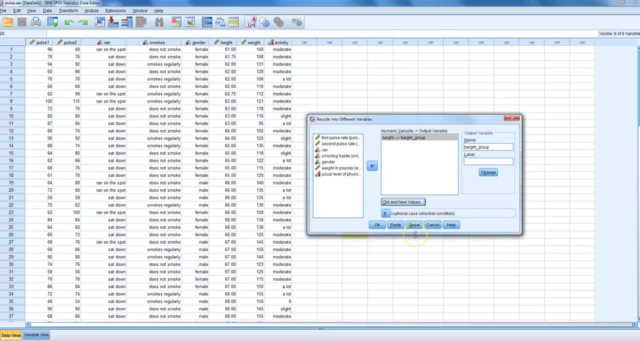 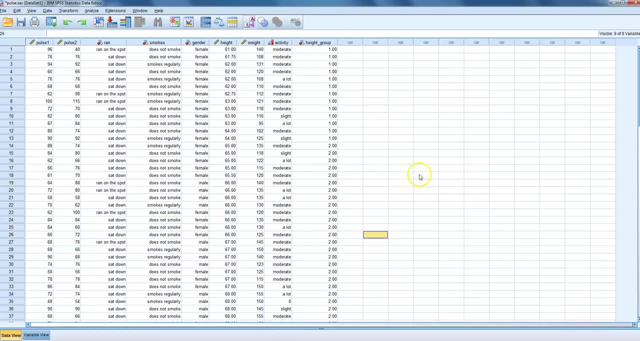 Select add and continue. Then we select OK. If we go back to the data set, we will see that a new variable has appeared. Those short people are put into group one, Medium people are put into group two and the taller people are put into group three.